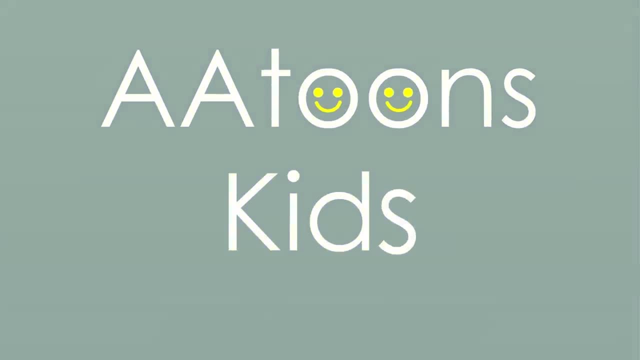 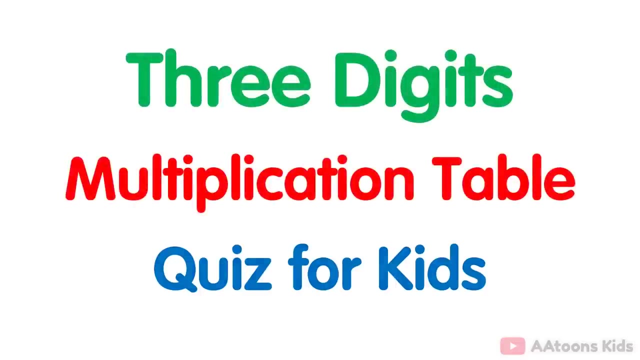 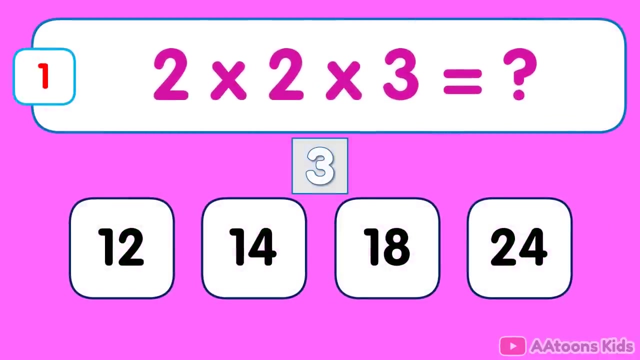 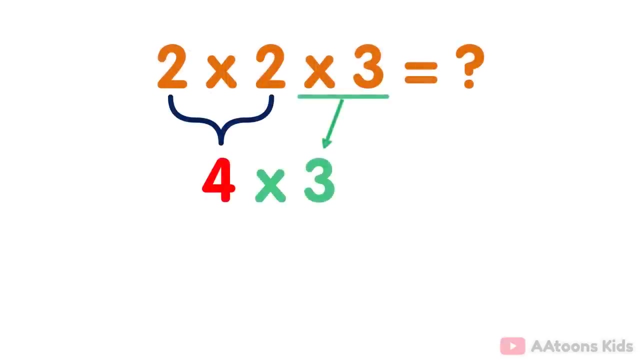 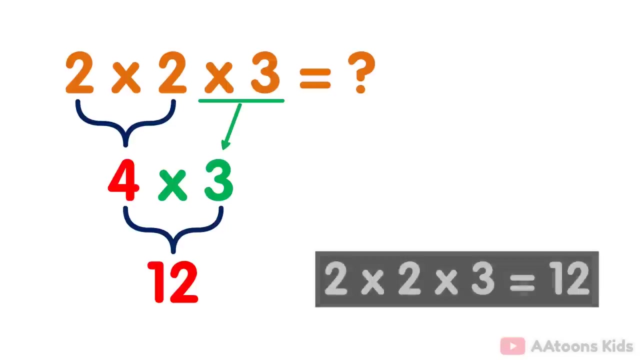 3-digits multiplication table quiz for kids. 2 x 2 x 3, 12. Simply multiply the numbers 2 and 2,, which equals 4.. Then you multiply the result 4 by 3. You will get 12.. Therefore, the answer to 2 x 2 x 3 is 12.. 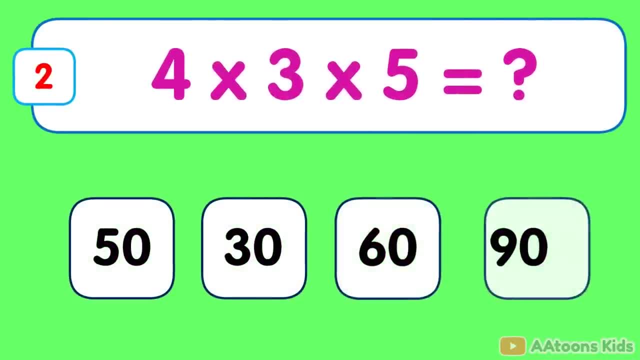 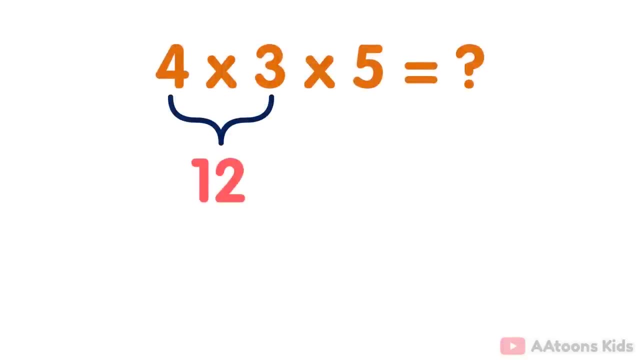 4 x 3 x 5: 60. Simply multiply the numbers 4 and 3, which equals 12.. Then you multiply the result 12 by 5. You will get 60. Therefore, the answer to 4 x 3 x 5 is 60.. 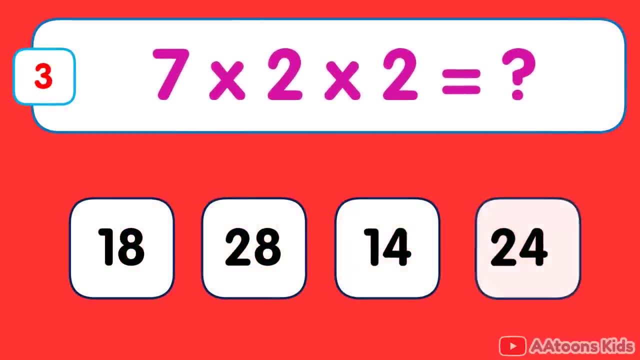 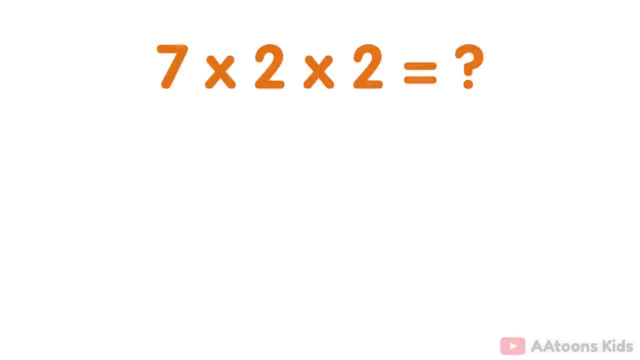 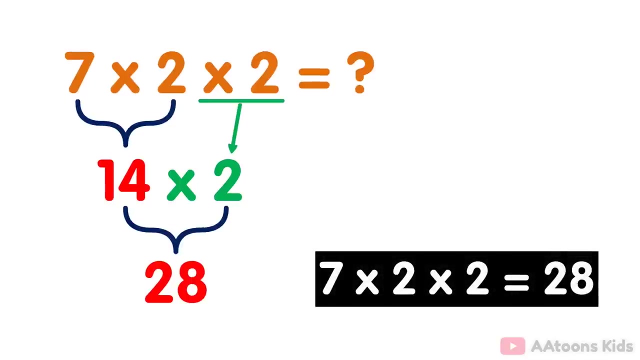 7 x 2 x 2. 7 x 2 x 2. 7 x 2 x 2. 7 x 2 x 3: 28. Simply multiply the numbers 7 and 2, which equals 14.. Then you multiply the result 14 by 2. You will get 28.. Therefore, the answer to 7 x 2 x 2 is 28.. 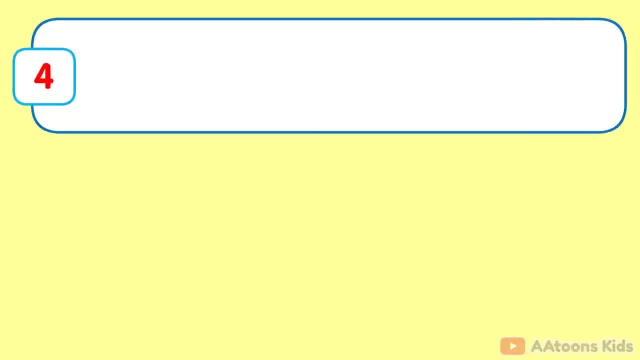 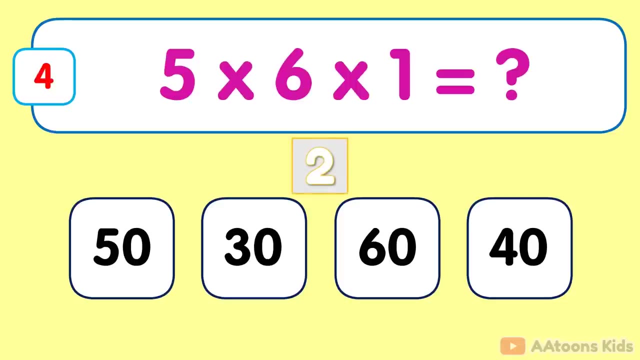 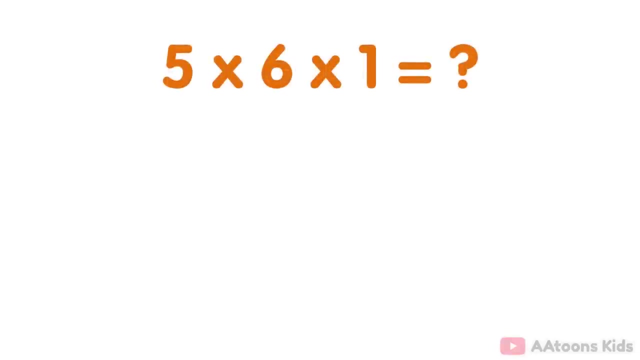 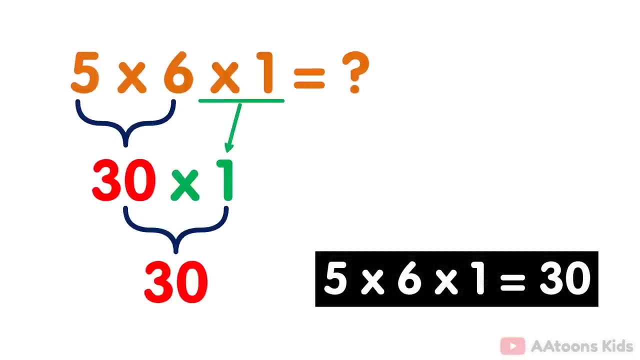 5 multiplied by 6, multiplied by 1, 30. Simply multiply the numbers 5 and 6, which equals 30. Then you multiply the result 30 by 1, You will get 30. Therefore, the answer to 5 multiplied by 6 multiplied by 1 is 30. 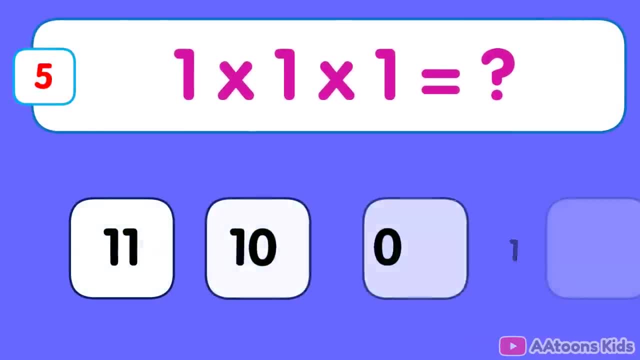 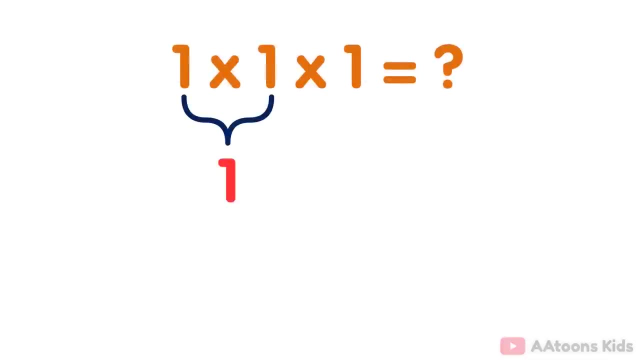 1 multiplied by 1. multiplied by 1: 1. Simply multiply the numbers 1 and 1, which equals 1. Then you multiply the result 1 by 1, You will get 1. Therefore, the answer to 1 multiplied by 1 multiplied by 1 is 1. 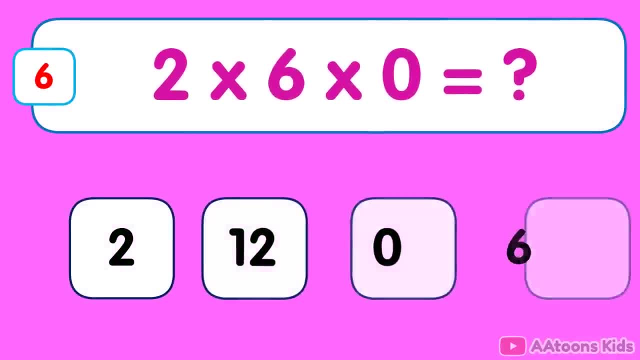 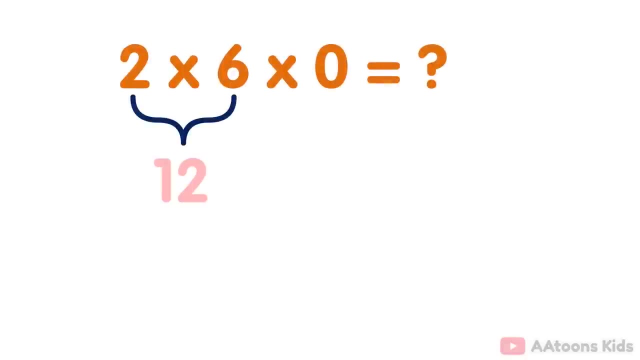 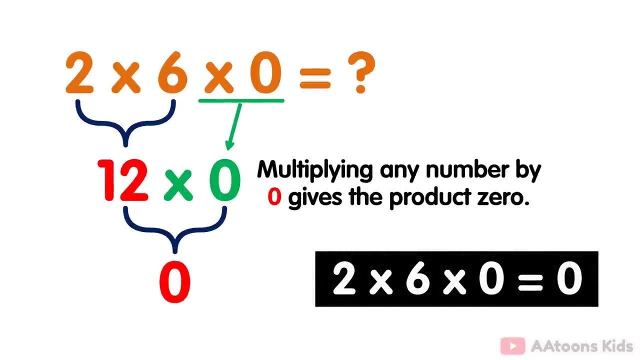 2 multiplied by 6 multiplied by 0: 0. Simply multiply the numbers 2 and 6, which equals 12. Then you multiply the result 12 by 0. Multiplying any number by 0 gives the product 0. Therefore, the answer to 2 multiplied by 6 multiplied by 0 is 0. 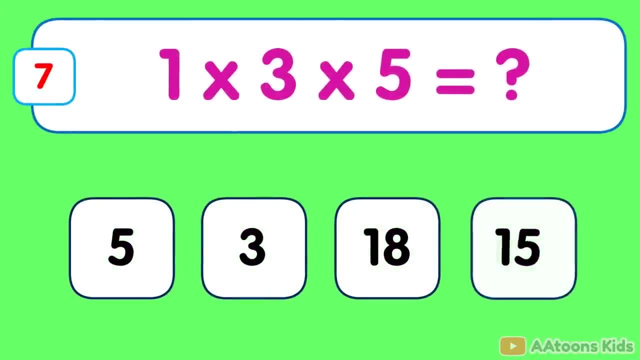 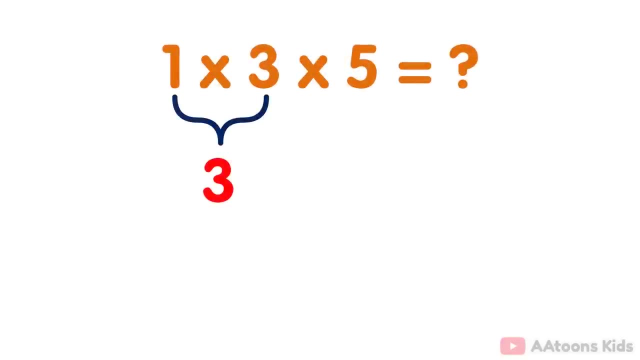 1 multiplied by 3, multiplied by 5, Then you multiply the result 3 by 5, You will get 15, 15. Simply multiply the numbers 1 and 3, which equals 3, Then you multiply the result 3 by 5, You will get 15. 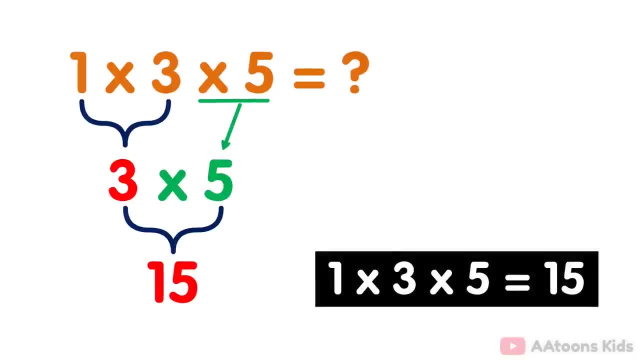 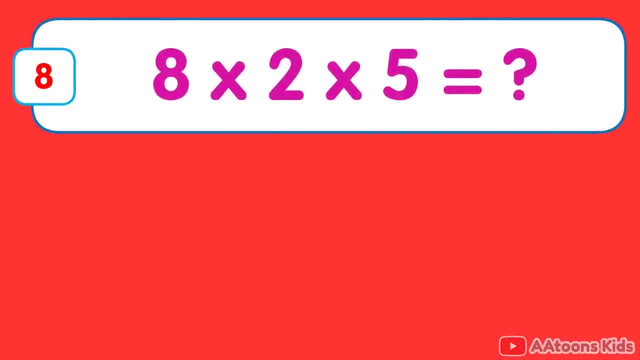 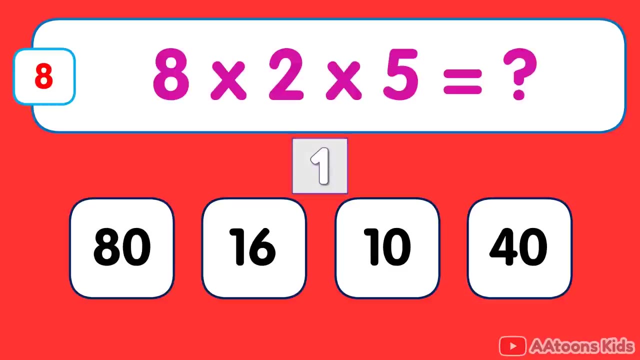 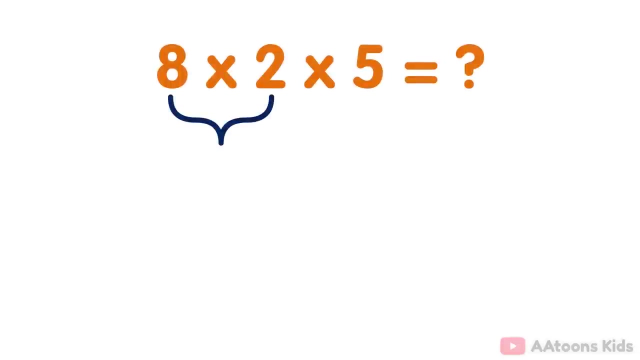 Therefore, the answer to 1 multiplied by 3, multiplied by 5, is 15, So you can get 16. So the answer to 1 multiplied by 3 is 5 multiplied by 4. You can find the answer in the description below: 8 multiplied by 2 multiplied by 5. 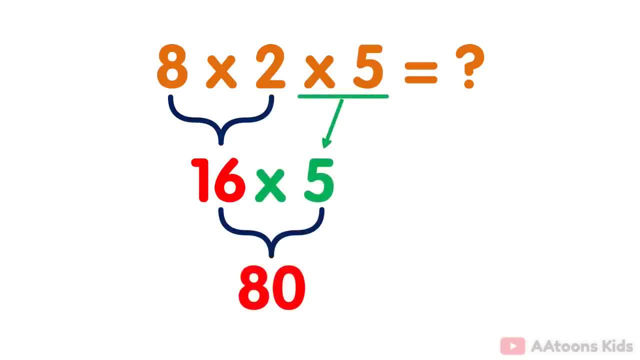 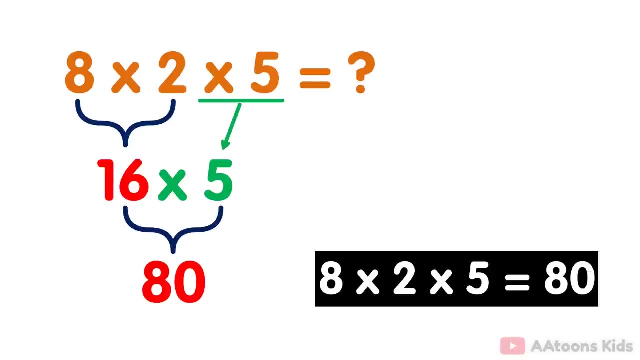 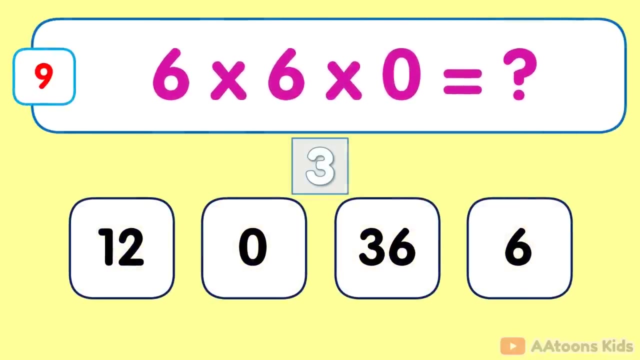 8 multiplied by 2 multiplied by 5 börjar. Therefore, the answer to 8 multiplied by 2 multiplied by 5 is 80.. 6 multiplied by 6 multiplied by 0: 0, Simply multiply the numbers 6 and 6, which. 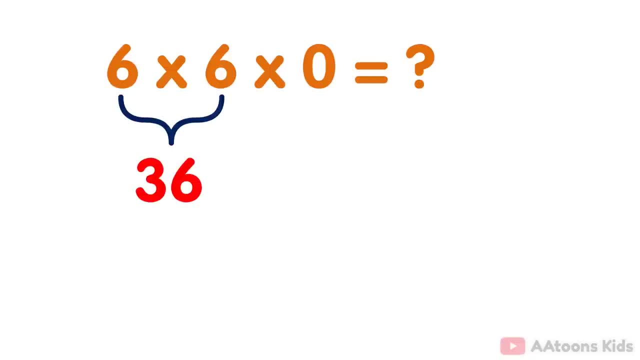 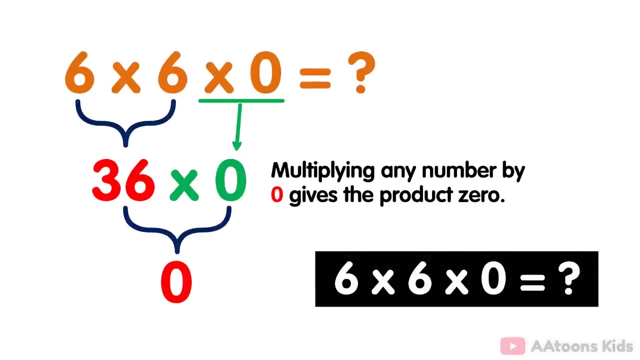 equals 36, Then you multiply the result 36 by 0.. Multiplying any number by 0 gives the product 0. Therefore, the answer to 6 multiplied by 6, multiplied by 0, is 0.. 8 multiplied by 0 multiplied by 5, 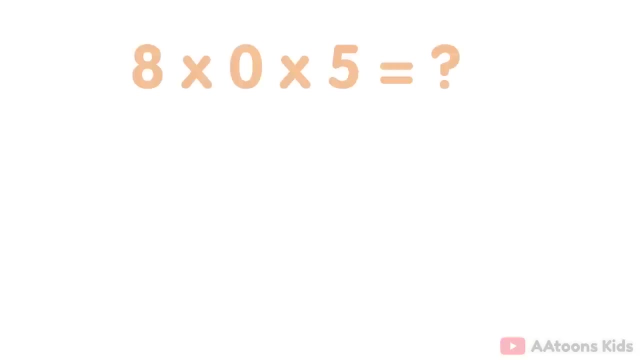 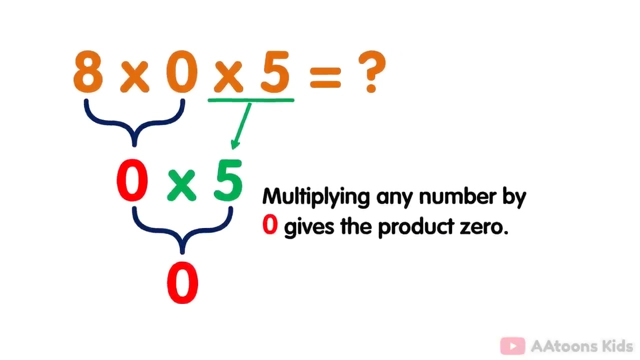 0. Simply multiply the numbers 8 and 0, which equals 0. Then you multiply the result 0 by 5.. Multiplying any number by 0 gives the product 0. Therefore, the answer to 8 multiplied by 0, multiplied by 5, is 0.. 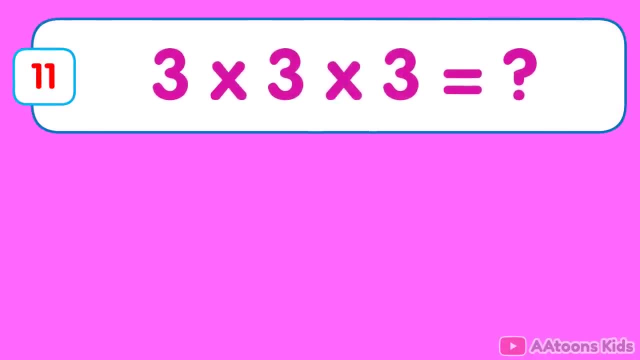 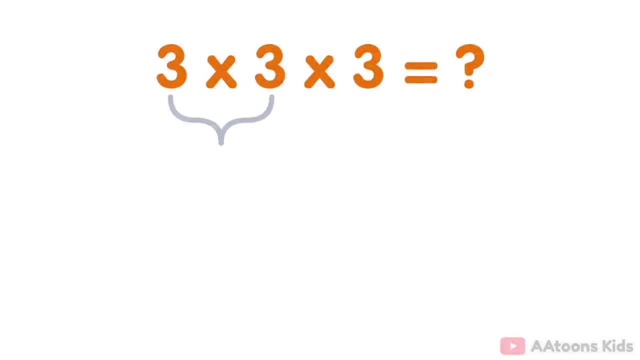 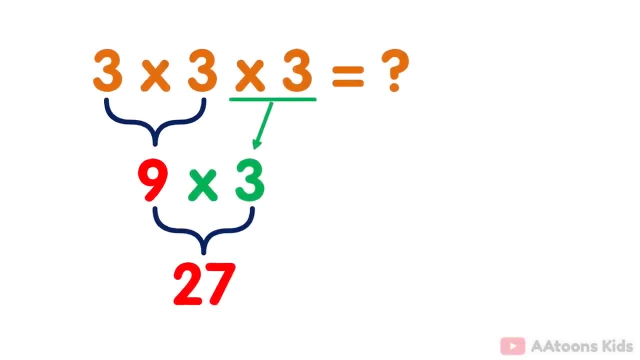 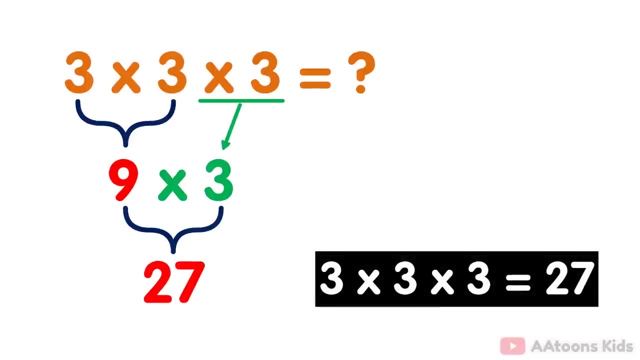 Then you multiply the result 9 by 3.. You will get 27.. Therefore, the answer to 3 multiplied by 3, multiplied by 3, is 27.. 5 multiplied by 4, multiplied by 3, multiplied by 3, multiplied by 2, multiplied by 3 multiplied. 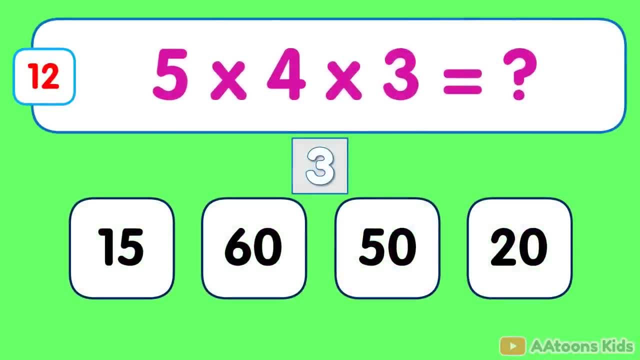 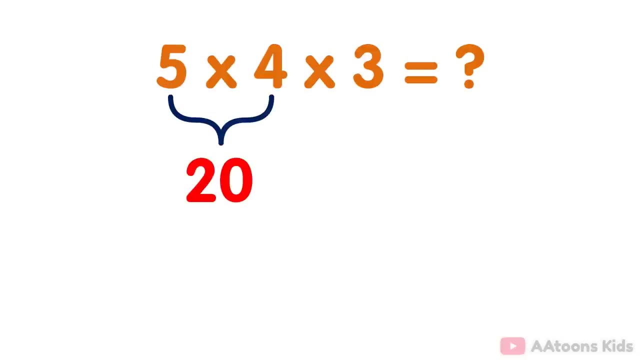 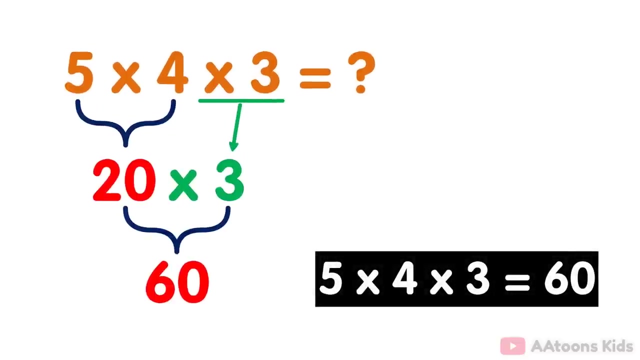 multiplied by 3.. 60.. Simply multiply the numbers 5 and 4, which equals 20.. Then you multiply the result 20 by 3. You will get 60. Therefore, the answer to 5 multiplied by 4 multiplied. 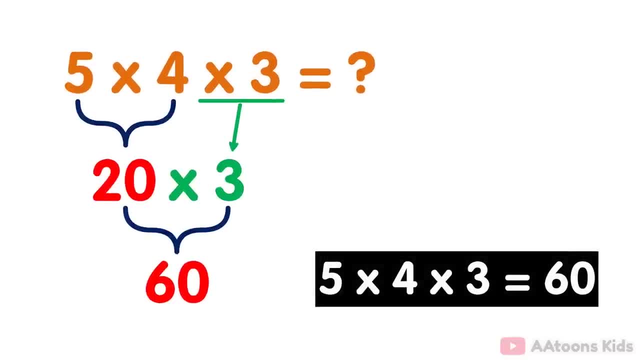 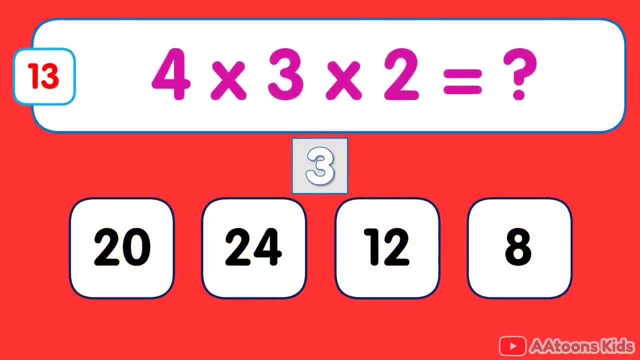 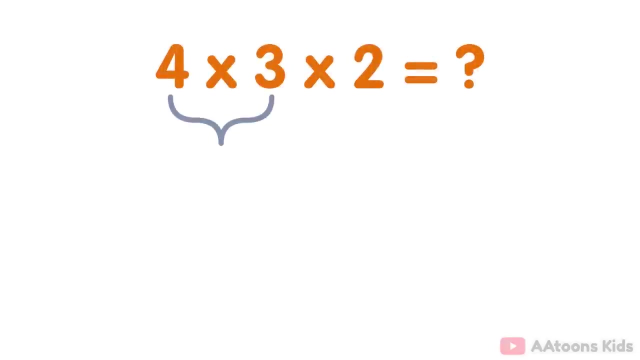 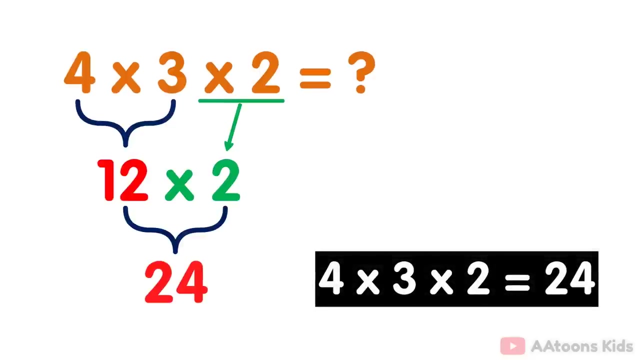 by 3 is 60.. 4 multiplied by 3, multiplied by 2. 24.. Simply multiply the numbers 4 and 3, which equals 12.. Then you multiply the result 10.. 12 by 2, you will get 24.. Therefore, the answer to 4 multiplied by 3, multiplied by 2, is 24.. 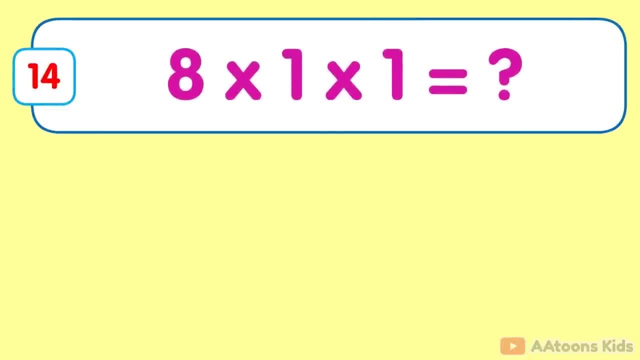 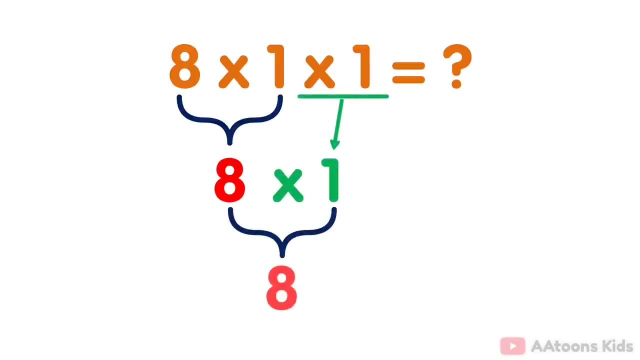 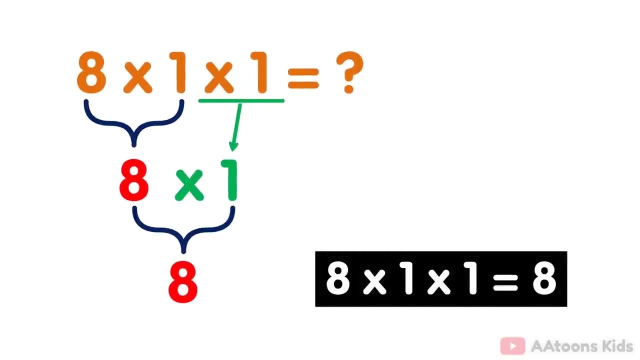 8 multiplied by 1, multiplied by 1.. 8. Simply multiply the numbers 8 and 1, which equals 8.. Then you multiply the result 8 by 1.. You will get 8.. Therefore, the answer to 8 multiplied by 1, multiplied by 1 is 8.. 2 multiplied by 4 multiplied by 6.. 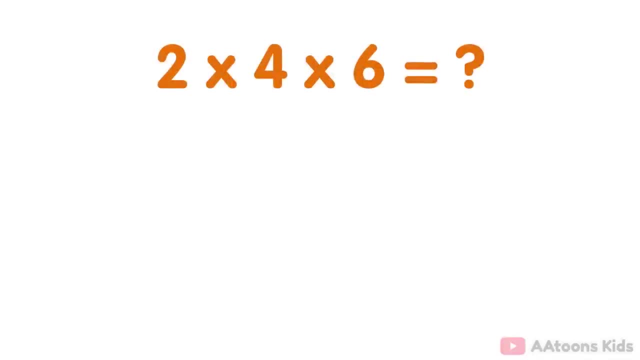 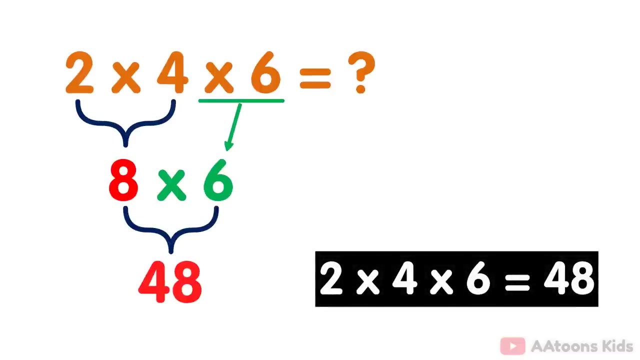 48.. Simply multiply the numbers 2 and 4, which equals 8.. Then you multiply the result 8 by 6.. You will get 48. Therefore, the answer to 2 multiplied by 4, multiplied by 6, is 48.. 4 multiplied by 3, multiplied by 4.. 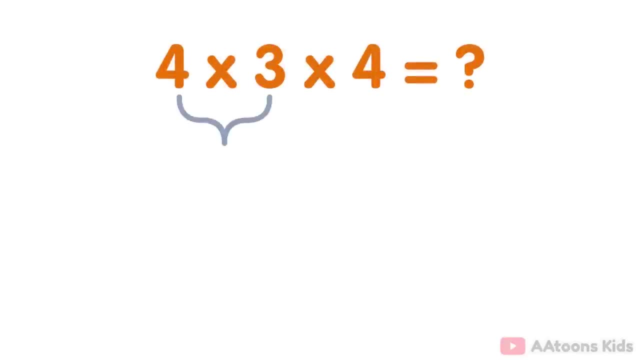 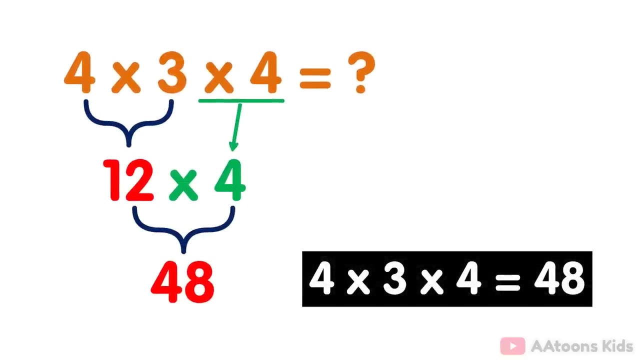 48.. Simply multiply the numbers 4 and 3, which equals 12.. Then you multiply the result 12 by 4.. You will get 48.. Therefore, the answer to 4 multiplied by 3, multiplied by 4, is 48.. 9 multiplied by 3 multiplied. 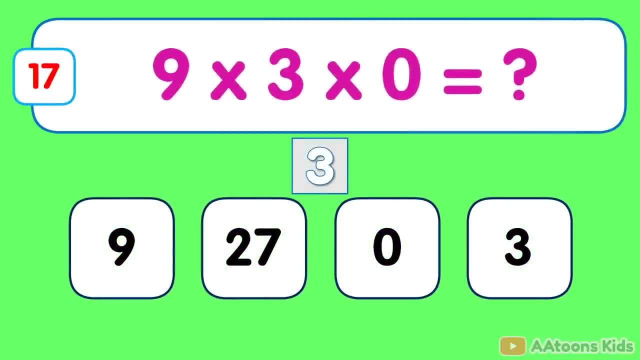 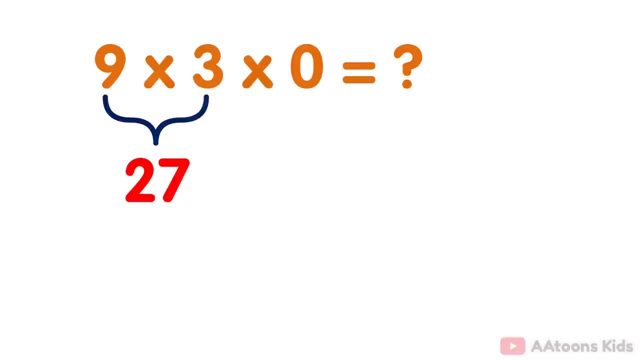 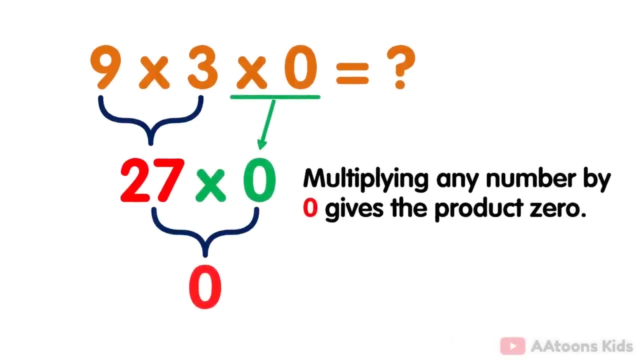 by 0.. 9 multiplied by 3 multiplied by 0.. OK, Simply multiply the numbers 9 and 3, which equals 27.. Then you multiply the result 27 by 0.. Multiplying any number by 0 gives the product 0. 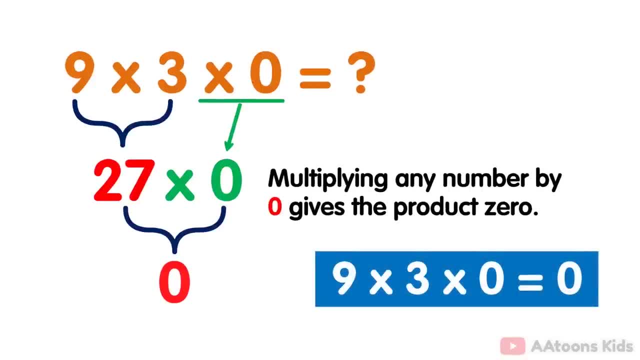 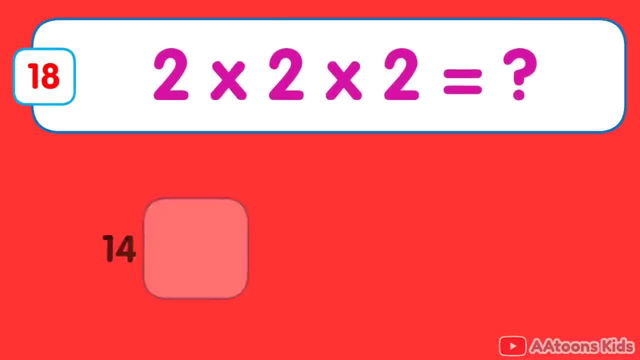 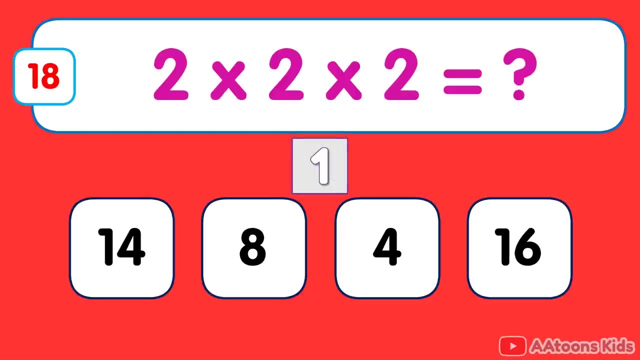 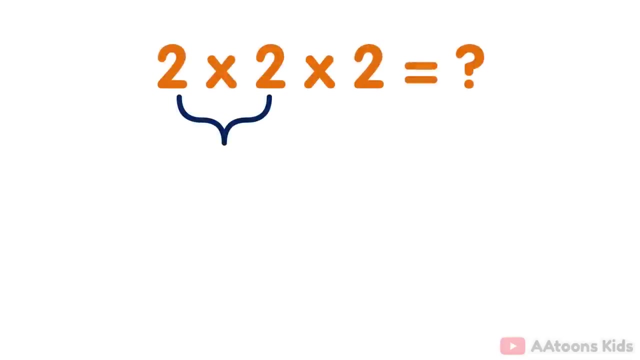 Therefore, the answer to 9 multiplied by 3, multiplied by 0, is 0.. 2 multiplied by 2, multiplied by 2, is 8.. Simply multiply the numbers 2 and 2, which equals 4.. Then you multiply the result 4 by 2..